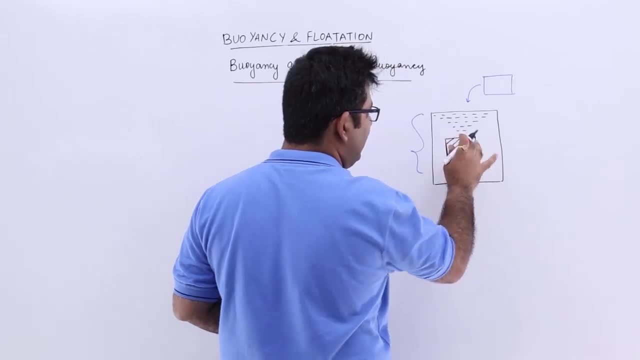 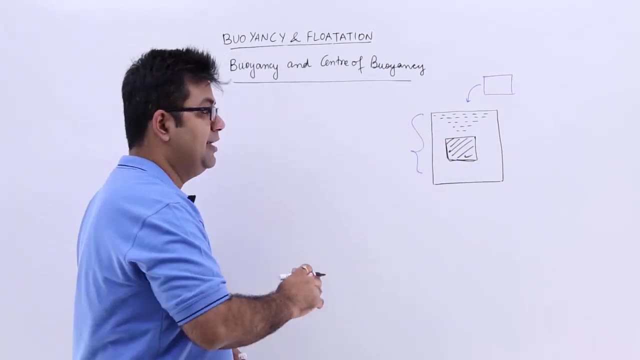 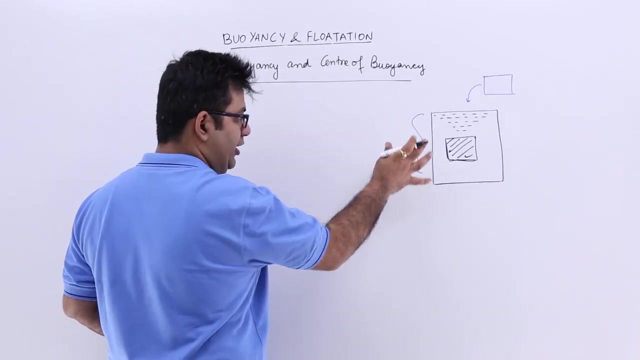 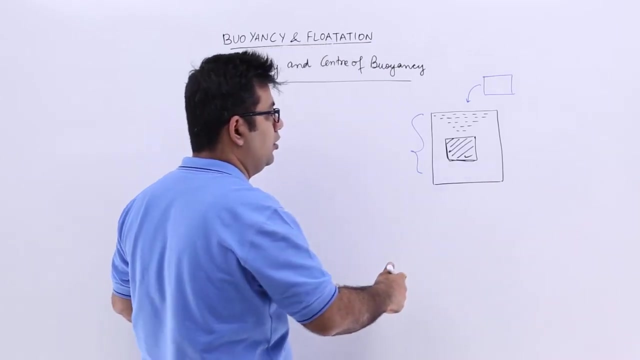 was taken out, which is equal to the volume of this entire body. So the volume of this entire body which has to come into this tank. An equal amount of volume of water has to be taken out. So this means when a body is put inside a liquid, there is an equal amount of, or you can say, an equal amount of volume. 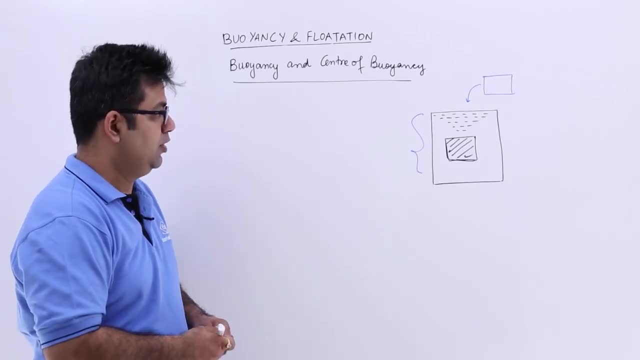 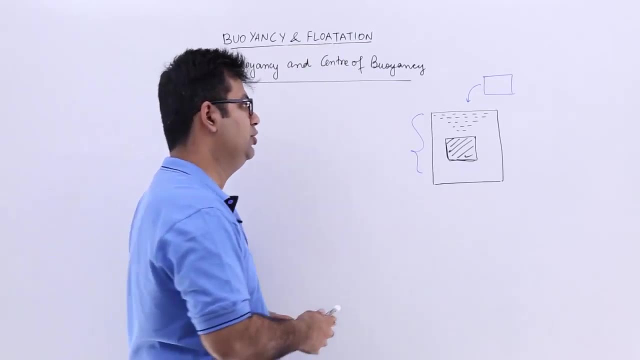 of liquid which is displaced by that body. Now, due to this condition, the liquid exerts a vertically upward force on this body. So this is the liquid which is displaced by this body. Now, due to this condition, the liquid exerts a vertically upward force on this body. 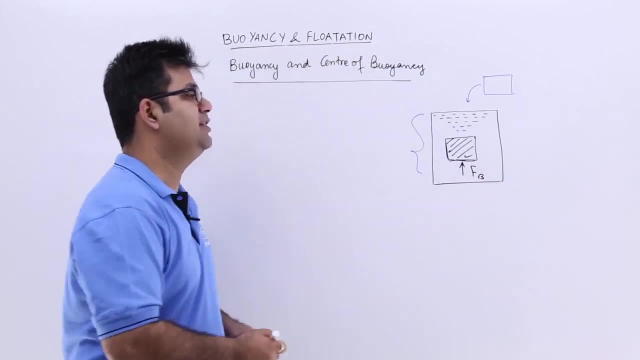 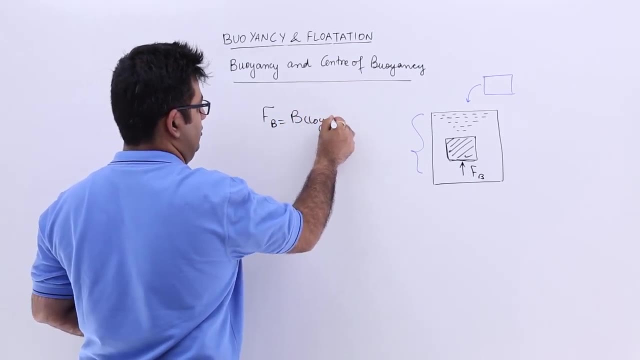 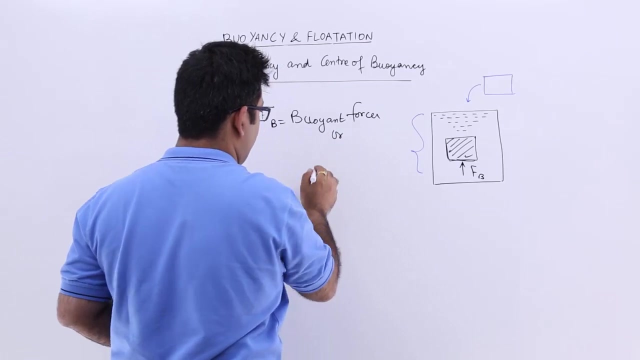 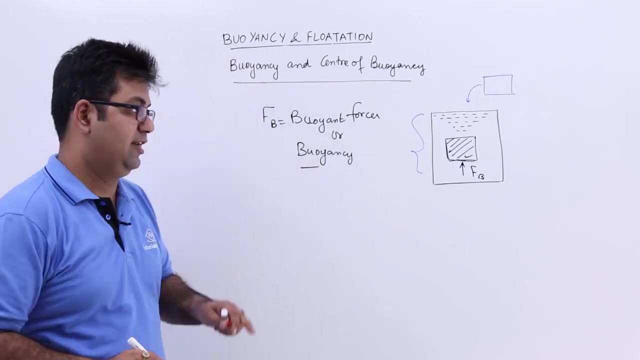 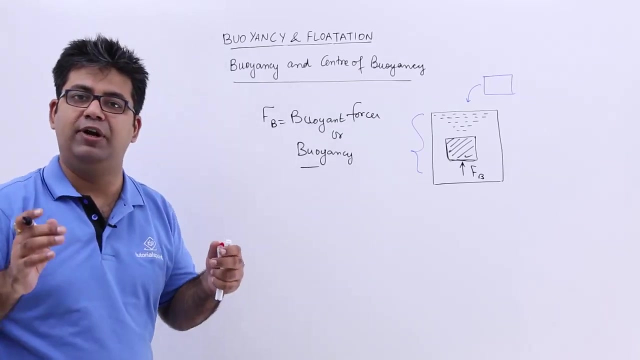 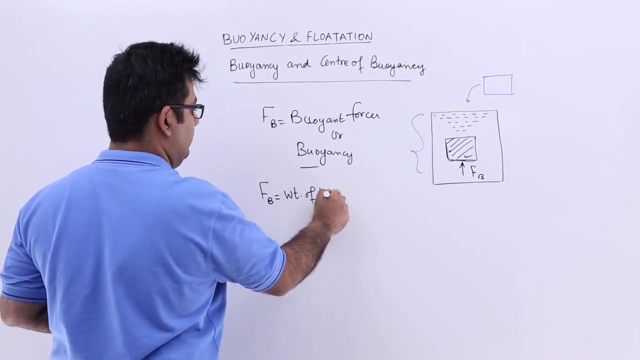 Like this And I denote that as FB. So FB over there is called the buoyant force Or simply buoyancy. Remember this is the force by the liquid onto the body, the magnitude of this buoyant force: this buoyant force is equal to the weight of the body. okay, 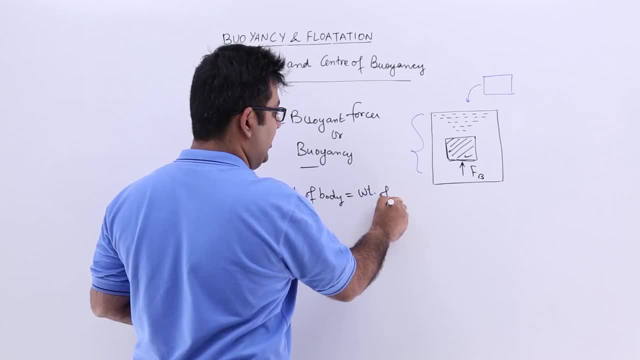 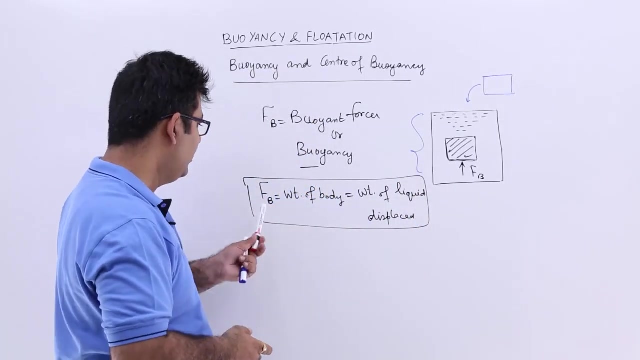 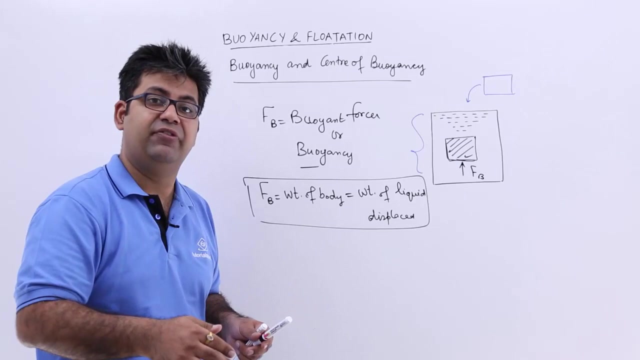 which is further equal to the weight of liquid displaced. okay, so you have to remember this concept, that is, the amount of buoyant force acting on the body by the liquid is equal to the weight of the body, which is further equal to the weight of the liquid displaced. because i told 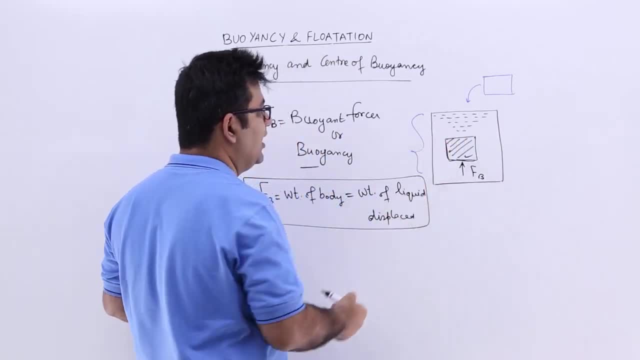 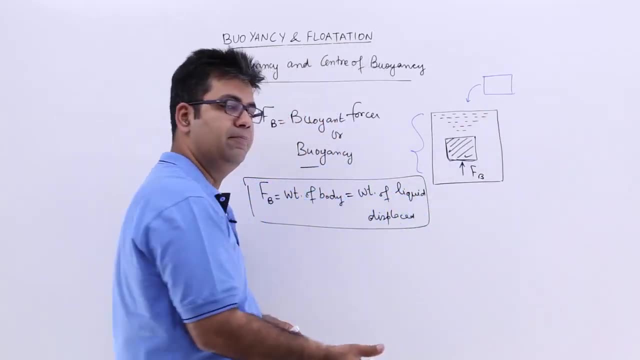 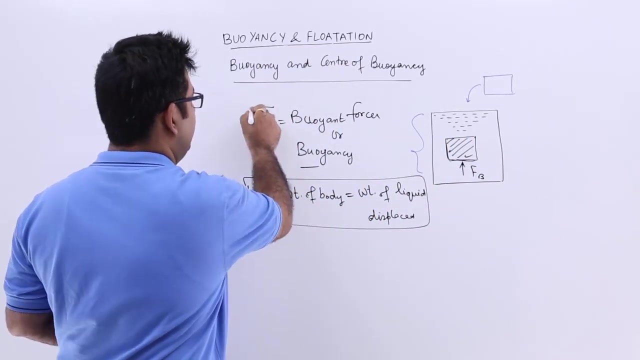 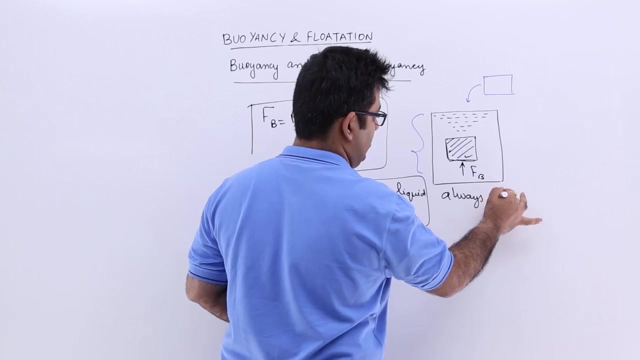 you that to keep this entire tank constituency as same as before, you have to take out some weight of the liquid and then only this block or this body would fit in. okay, so that is the concept of the buoyant force. buoyant force, which is an upward force. always remember this is always upwards force. okay now. 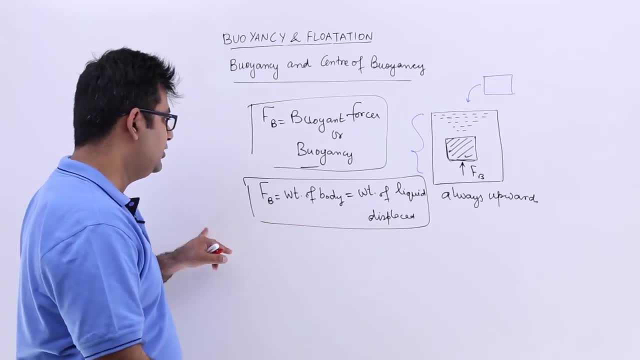 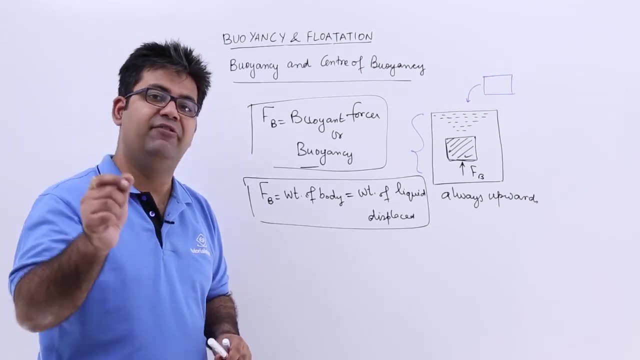 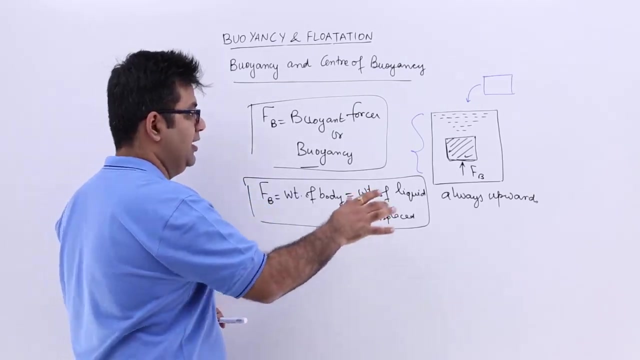 the magnitude i have also told you is equal to the weight of the body or equal to the weight of the liquid displaced. now you must always remember that the weight of the body acts through the center of gravity of the body, but the buoyant force, it always acts.